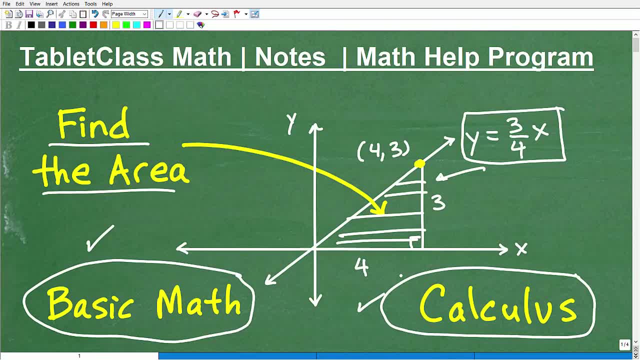 So we're going to go ahead and find the area of the base of 4.. But we're going to show you here- or I'm going to show you- exactly how we can use calculus as well- to find the area of this triangle. And the work is not. it's a couple more steps than using this basic formula right here, But it's not that difficult. So really, the whole main idea of this video is not to find the area of a triangle. I mean, this is a good little review for that as well, But it's just to give you an appreciation of the power and usefulness of calculus. Okay, now we're not going to want to use calculus. 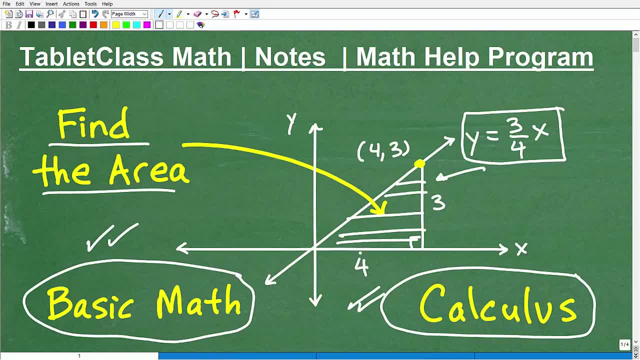 We're going to want to use calculus to find areas of triangles, But I'm going to show you how we can use calculus to find the area of all kinds of crazy objects that you might encounter where you may not have a formula handy. So we're going to talk about all this in just one second. But first let me quickly introduce myself. My name is John. I'm the founder of Tablet Class Math. I'm also a middle and high school math teacher And over several years I've constructed what I like to believe is one of the best online math help programs there is. Of course, I'll let you be the judge of that If you're interested in. 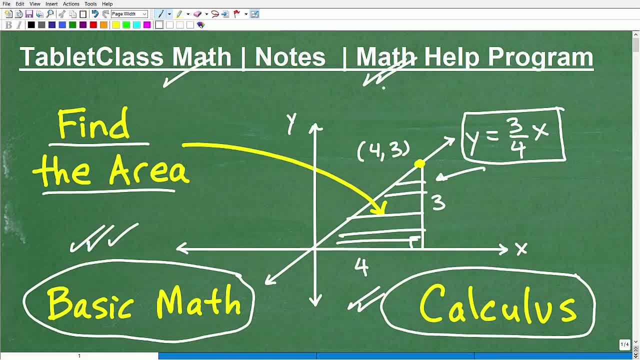 my math help program by following the link in the description of this video. But basically I have 100 plus different math courses, ranging from pre-algebra, algebra 1, geometry, algebra 2.. I'm going to be launching pre-calculus here very, very soon, in a matter of a few weeks. So that's you know. I love advanced mathematics So I can't wait to get that course out there. But I also have many courses in the area of test preparation. So if you're studying for like the GED, SAT, ACT, GED, etc. 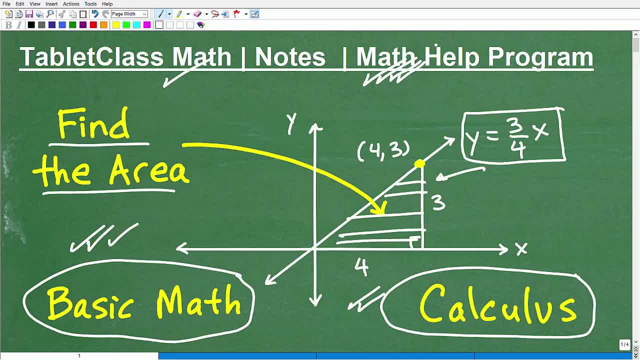 GRE, GMAT, ASVAB, ACCUPLACER, ALEC test, CLEP exam, maybe a teacher certification exam, maybe a nursing school entrance exam like the TAS- Any of those exams, or all those exams or many others, have significant math on the exam. So people have to take these exams or take certain exams for all kinds of reasons to get to where they want to go in life. But if you don't do well, 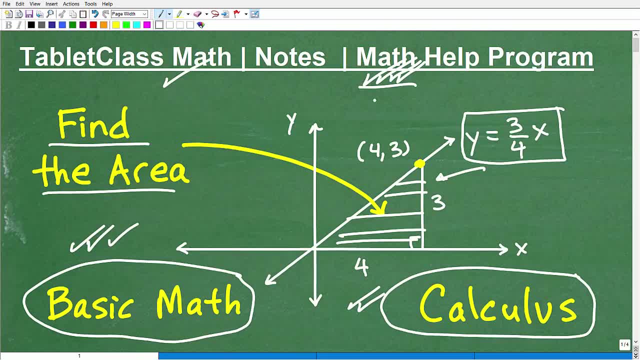 on the math section. you don't do well on exams, So let me help you prepare. Just go to my website, check out my full course catalog. I should have what you're studying for If I do not. drop me a line and I'll help you out the best I can. I also do a lot with independent learners, like homeschoolers. So if you homeschool- I have a great homeschool learning program and working with homeschoolers for 15 plus years- Then obviously I help those of you that are just having a tough time in your current math courses. Now, if you truly are serious about wanting to improve or learn mathematics, then you must be serious about this and that. 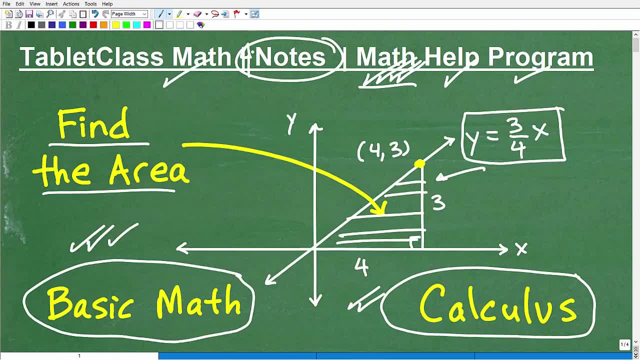 That is note taking, OK. so over decades of teaching math, it's apparent to me that those students who take the time and effort on a daily basis to take great math notes, they almost always do very, very well, And that's not surprising. And then the reverse is true. Those students who like to look at their cell phone, talk to their buddies in class and maybe do their homework for another class during math class- All the stuff that I did way back in the 1980s, except for the cell phone part- none of our- myself or anyone else. 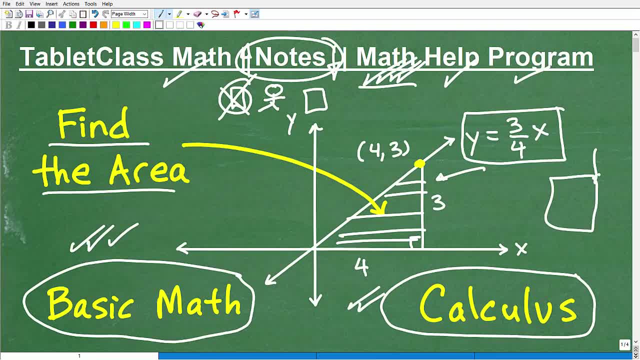 Had cell phones. By the way, those cell phones were like huge. They were like, you know, the size of a book and they cost like five thousand dollars. But I don't want to digress too far down memory lane. And of course he couldn't do anything fancy. Maybe you could. I don't know if you could have text or whatnot, But nevertheless we were. I was certainly distracted and my grades reflected that. OK, so they weren't good. So the bottom line is this: If you truly are serious about wanting to do well in math, you have to take great notes. All right. So just, there's no shortcuts. 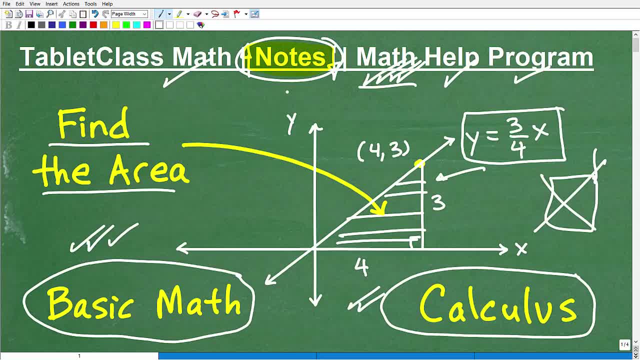 If there was, I certainly would tell you that, or tell you those little hacks and tricks and shortcuts, But unfortunately there isn't. when it comes to note taking Now, as you're improving in your notes, you still need something to study from. 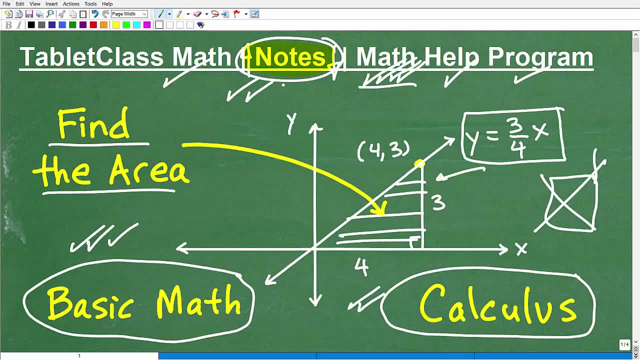 So I offer detailed, comprehensive math notes to include pre-algebra, algebra and geometry, algebra to and trigonometry. You can find the links to those notes in the description of this video. All right, So let's get into this triangle problem again. We want to find the area of this triangle right here. 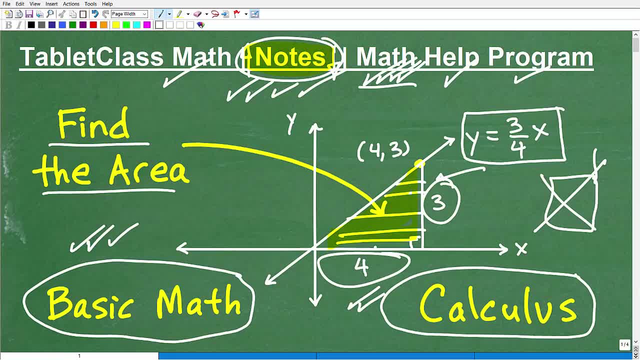 It's height is three. Its base is four. So if you think you remember the formula, go ahead and quickly do it. Do the calculations. I'm going to go ahead and do this right now. So if you don't want to see the solution just yet, pause the video. But let's get to it. 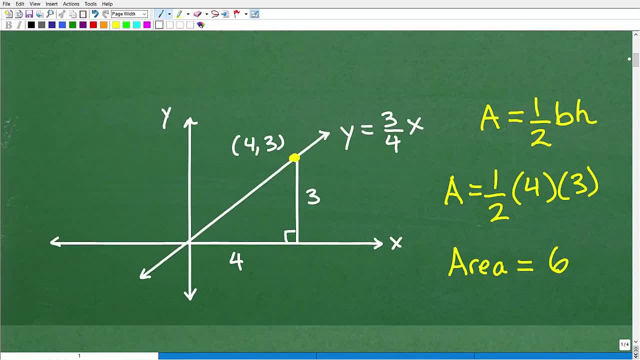 All right. So here is basic math. So to find the area of this triangle, we need to know the formula for an area of your triangle. OK, luckily we have one, And here it is right, here in its glory. The area of a triangle is equal to one half the base times height. Now, depending on the kind of the orientation of the triangle, we'll have to figure out what the base and height is. 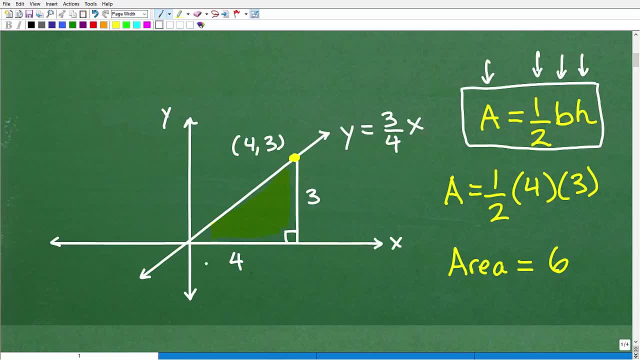 But this particular one. this is a nice lovely right triangle So we can look at four as the base and three as the height. So we literally just plug in those values. So the area is going to be one half base, which is four, And the height is three. So one half times four times three is twelve, Twelve, One half of twelve is six. 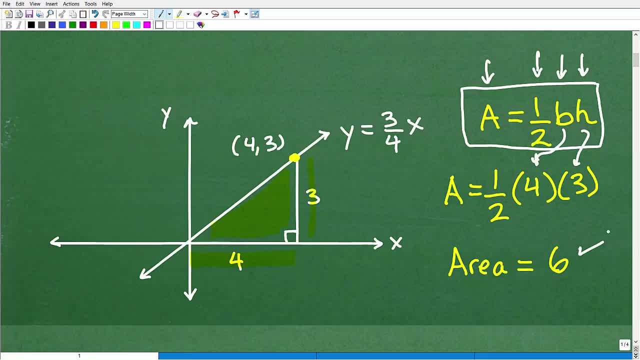 So the area of that triangle is six, And that is that OK. so you know, if you got six, then I must give you a nice little happy face with a checkmark. Now, that was super easy. But what was, you know, the key to doing this problem? Well, it was a formula, OK. 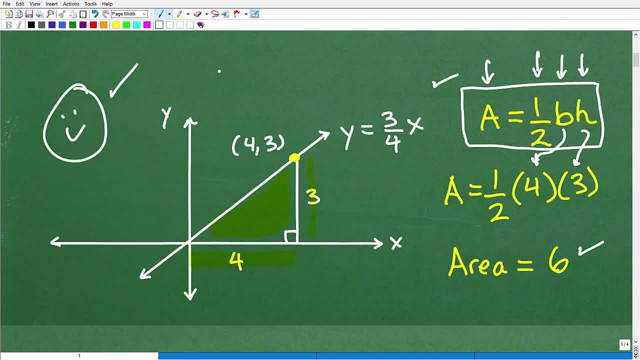 Formula for the area of a triangle. So you know, luckily, if you come across any triangle right, anything like this or whatever the case is, you can always use this formula, as long as you can determine the base and the height of those triangles. 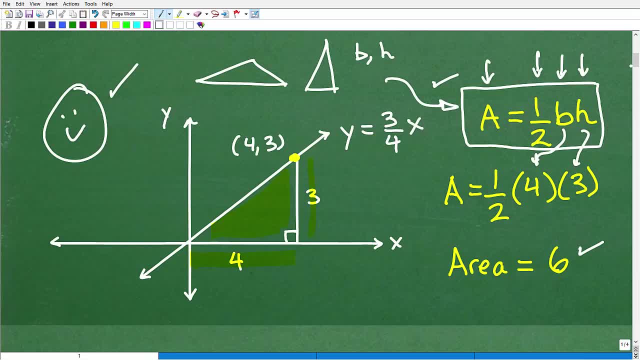 So that's awesome, All right, Now let's check out how we can use calculus Now. obviously, the area is six, So the answer is not going to change, But our approach is going to be completely different. So let's. 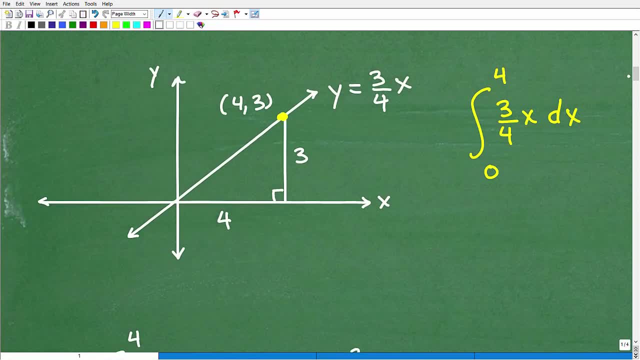 Show you how calculus works. All right Now. I've done quite a few videos on calculus and the essence of it, And my kind of goal in all those other videos, and this one as well, is just to show you the application of calculus. 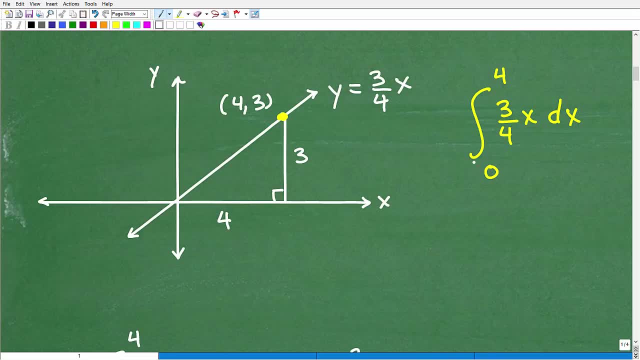 So, calculus, we have this crazy looking symbol right here. This little thing right here looks kind of like an S, Right? So S is the first letter, obviously, in the word sum, And this little thing is what we call an elongated S, So it's like an S stretched out. So we're really kind of finding the sum. But what we're going to be doing in calculus, we're going to be finding the area. 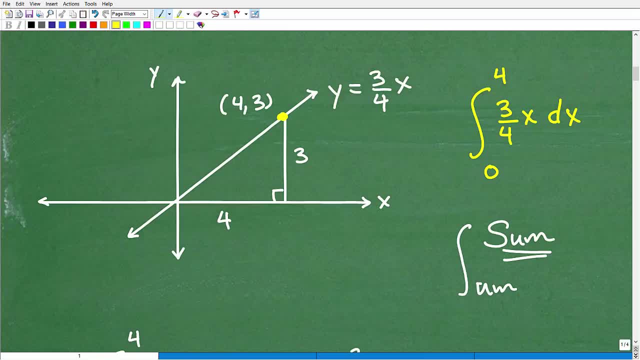 So this little thing is called an integral, or the symbol itself is called an elongated S. But basically what we're going to be doing is finding all these little, tiny little rectangles that can fit underneath here, because we can find the area of a rectangle and their rectangle is very easy. 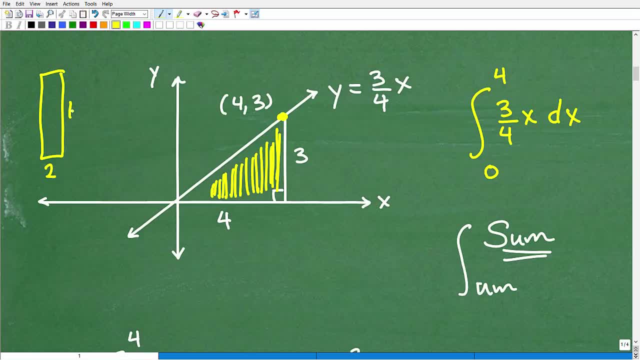 So let's say I have a rectangle. Its base is two and its height is 10.. What's the area of that? It's two times 10 is 20.. OK, so what we do in calculus is we find the area of all these little triangles that could fit underneath this. 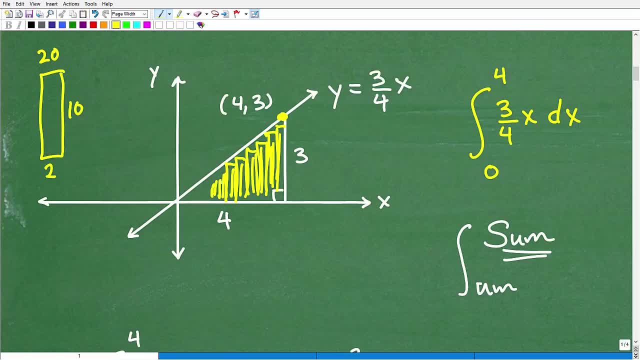 I'm sorry, the area of all these little rectangular strips, if you will, that can fit underneath this triangle. Now, if you have big, thick rectangles then our area Estimation is not going to be so good. But if we had like infinitely skinny little rectangles, we could have a precise Matter of fact, an exact OK. if we had infinitely skinny or little rectangles, we can have the exact area of this triangle. 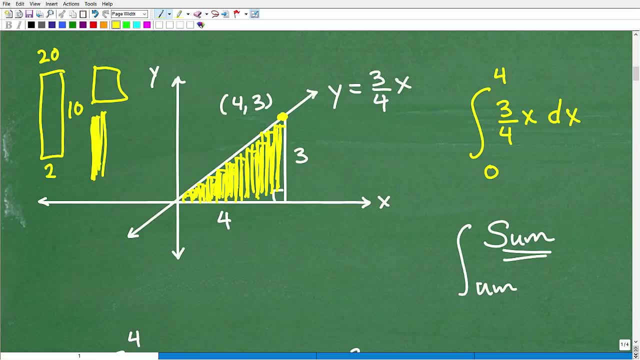 And that is effectively what calculus allows us to do. Now, some of you might be saying: well, why do I need to do all this crazy stuff right here? I don't want to do calculus. I'm like: yeah, You know, I want to take the easy way out, and I agree You should take the easy way out. However, I'm going to get to the mechanics of this particular problem here in a second. 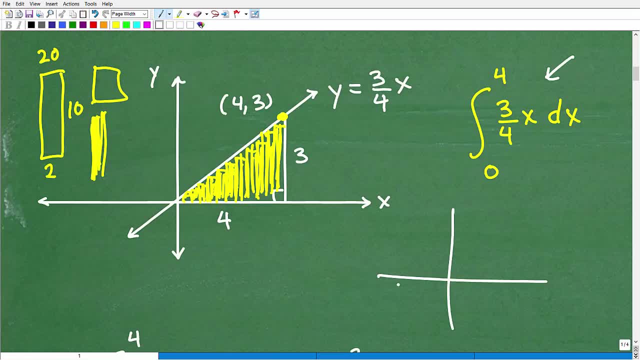 What if, instead of a triangle, what if we were trying to find the area of something like this? OK, so now we're looking at like this thing right here, And so some of you might be like, no problem, Give me the formula for the area of this. 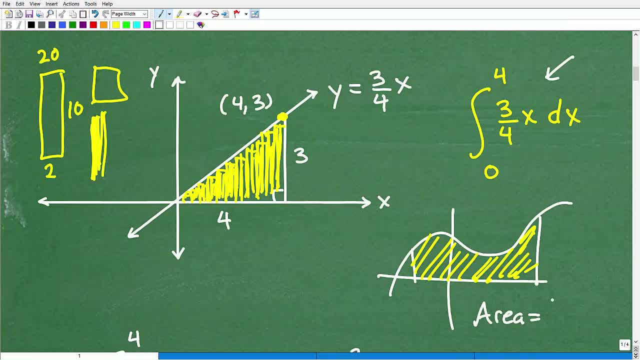 So I mean, I don't even know what we call this, right, Let's call it a thingamajiggy, right, A thingamajiggy. whatever the case is, I'll just abbreviate it. So you go in your math book and you look up: hey, what's the? 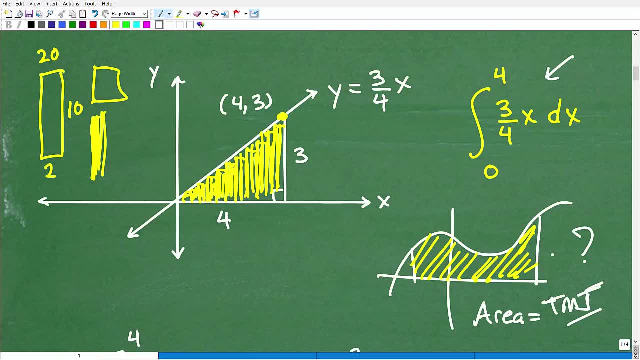 formula for a thingamajiggy And unfortunately there is no formula, okay, for this object. So you're like, oh, no formula. How am I going to do this? Well, calculus would be your, you know. 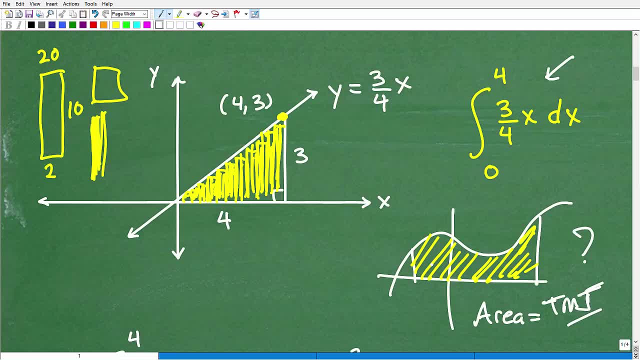 superpower right here. You need calculus in order to do this problem. okay, Now, obviously, we're going to. I'm going to show you how calculus works to find the area of this particular triangle. But the same technique- is what I'm going to show you right here- could be applied to find the area. 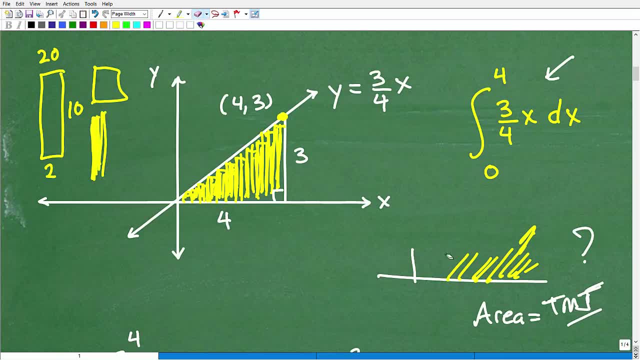 of this guy as well. It's obviously a little bit more challenging, The math is a little bit more involved, but not that much more involved. okay, But that's for another video, another time. So okay, so what do we do here? Well, here we have our little triangle. okay, Its base is four. 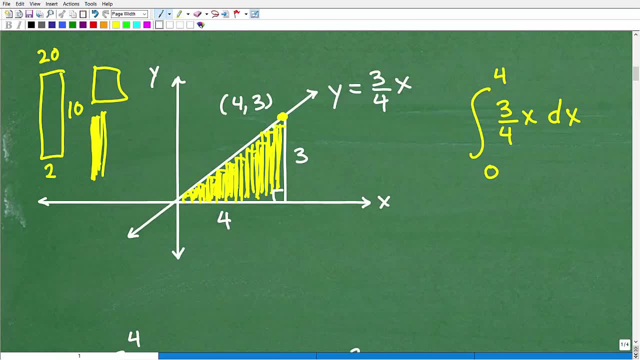 its height is three, But the, this, the hypotenuse, this part of the triangle, this is a line. okay. Now, if you understand, lines like y equals mx plus b, and I'm really kind of gauging this or gearing this video towards anyone. 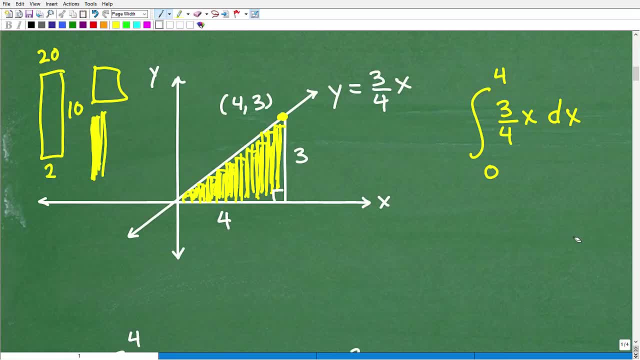 who's taken any kind of basic algebra, right. But even if you haven't taken any algebra, this little equation: y equals three-fourths. x is the equation for this line right here. okay, That's the the corner of this triangle. 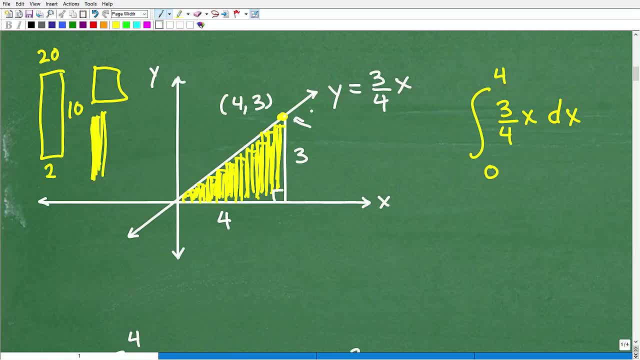 So in calculus we can write ourselves a little kind of prescription here of how to find the area. So we're going to say this little long s we're going to say, all right, we want to find all the little rectangles. okay, Like I just described here for this function, right here, three-fourths x. 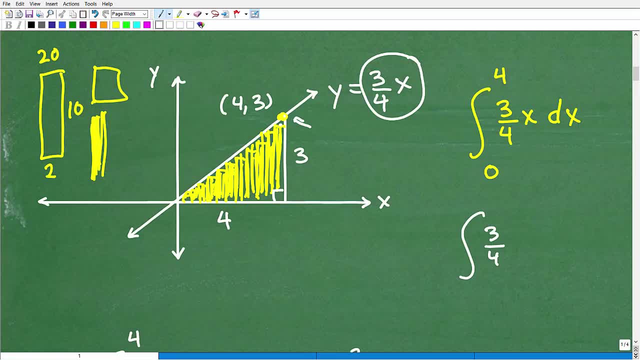 All right, So we want to find all the rectangles under this line, okay, and it borders the x-axis, and then we put a little x right there and this dx. that's just a little notation that we we use, but i want to count the rectangles from zero. this is zero, zero. 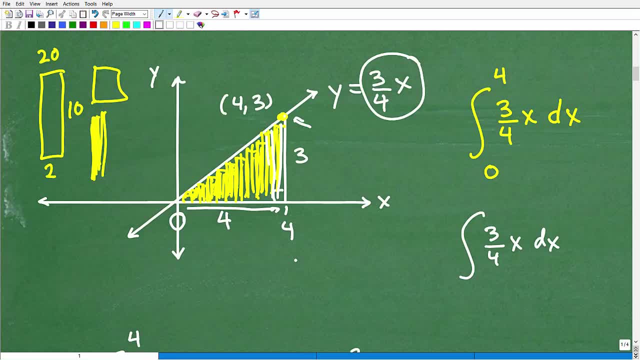 all the way out to four. okay, so i'm going to start from zero and i'm going to go to four. so that's how we find the area, okay, of this triangle, right. so we're basically uh kind of programming our little calculus notations like: all right, start from zero, go all the way out to four and find all. 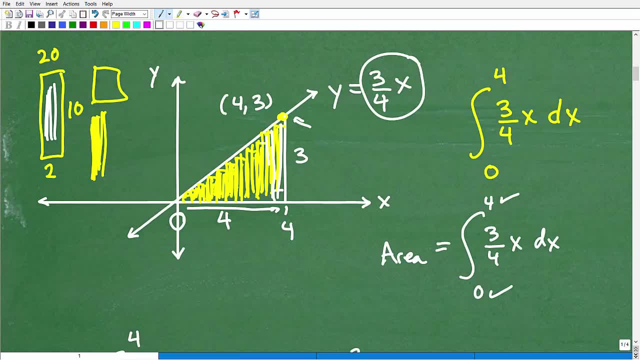 the little rectangular strips underneath this uh line, okay, this line right here, and this line, if you go straight down perpendicular, it forms a triangle. so i know, i'm kind of, i'm kind of keeping this very basic, but if you understand so far what i'm talking about, then that's excellent, okay. so 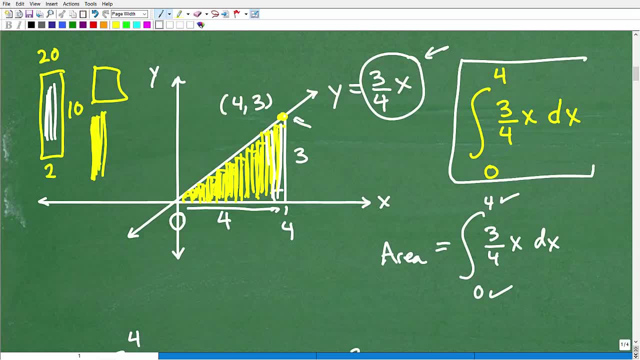 now what we have to do is do the mechanics of actually calculating this out. so we're going to have to solve this basic integral problem. so this is called integration in calculus. this is all and basically just means to add up, and effectively we're going to be doing is adding up all these. 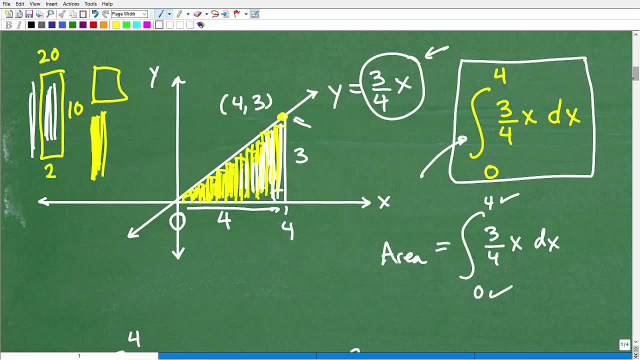 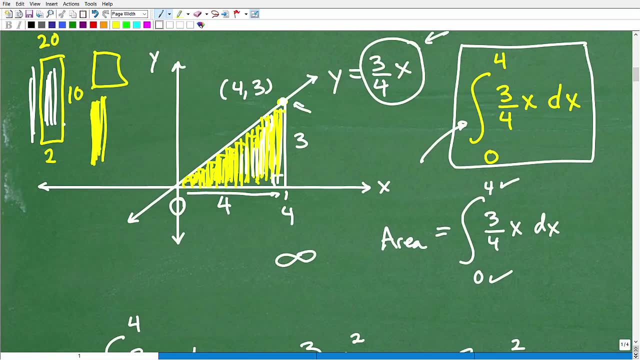 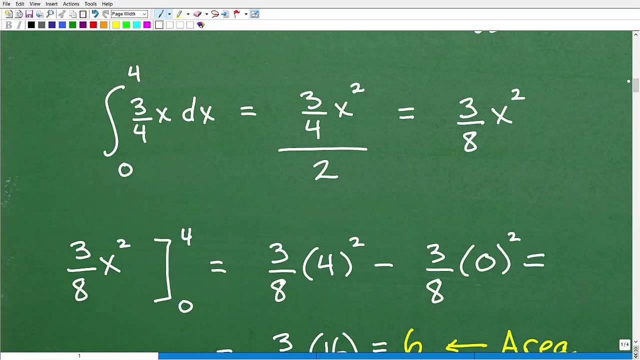 little, infinite tiny little rectangular strips. but, uh, we have some pretty easy way of adding this up. we're not going to have to do infinite amount of addition, okay, so, luckily, i'm going to show you this now. all right, so the first thing we have to do is we have to, uh, 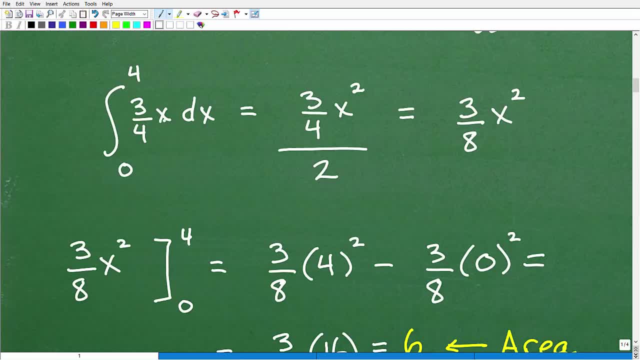 evaluate this integral, we have to find the integral of three-fourths x. okay, so don't worry about this notation. this isn't a formal calculus course, but basically i got to get rid of this little symbol here and i got to this symbol. this elongated s is integral three-fourths x. 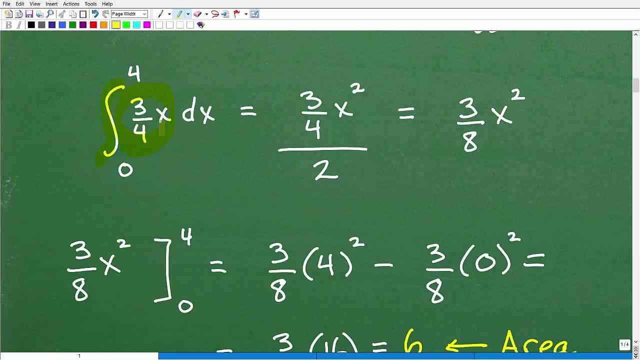 i have to do something with that. well, in calculus we actually have a formula and basically it states this: so this three-fourths x, this x here is really x to the first power. so i want you, i want you to do this part. so here is what the formula tells us in calculus. so that power one. see that little one. 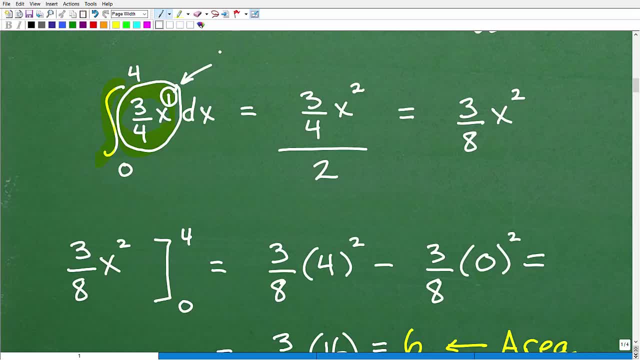 right there. okay, you add a one to it. it's always a one, okay, another. so if that was squared, we would still add a one. if this was like x to the fourth, we still add a one. so it's going to be one plus one, which is, in fact, what? two? okay, so we're going to write three-fourths x, we're going to increase. 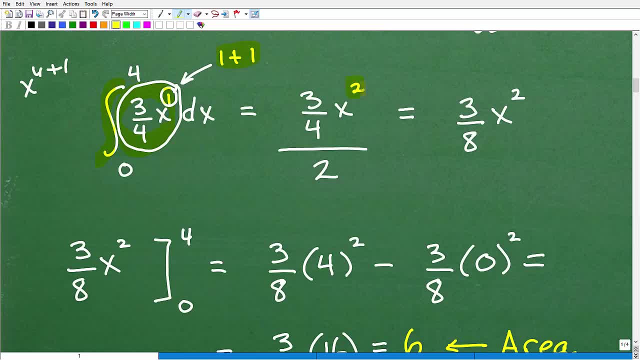 that little power by one, so that's going to be two. and then whatever that power turned out to be- in this case it's x to the second power. okay, you're going to divide by that little um, that exponent, so in this case it's two, so we're going to divide that. 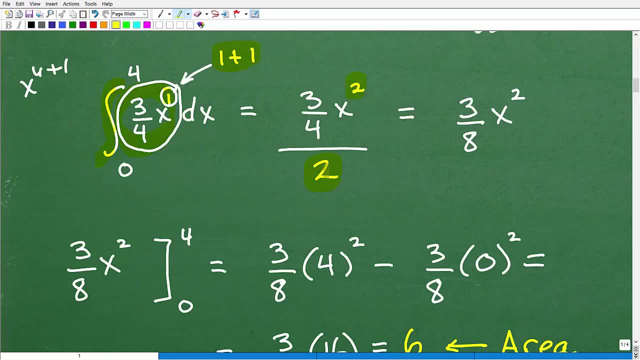 three-fourths x squared by two. okay, so if you understand that, you understand basic integration and calculus. now, um, this little x thing. this is a basic polynomial and there's all kind. there's different type of rules that we need to use, uh to uh find the 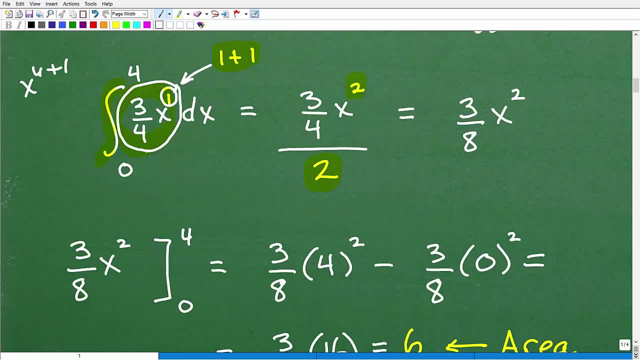 integral in calculus. but this is a very, very common uh rule, right here, right? but it's not difficult to follow, right? I mean so far. hopefully you know this isn't too scary. so now we have to figure out three-fourths x squared divided by two. okay, so three-fourths divided by two. when you do, 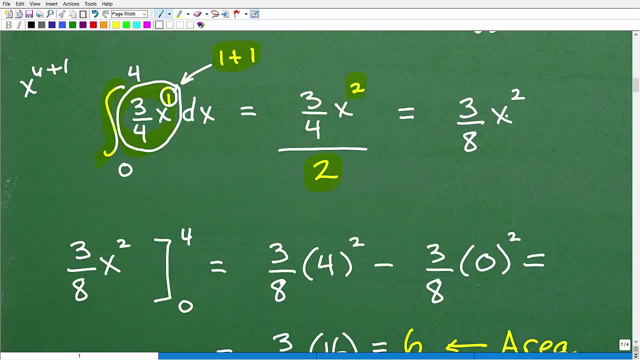 that lovely little fraction math, you will get three-eighths x squared, so just do the. let's do this real quick: three-fourths divided by two is equal to three-fourths times one-half, of course. by the way, if you have any trouble with fractions, I have a ton of uh videos about fractions on my 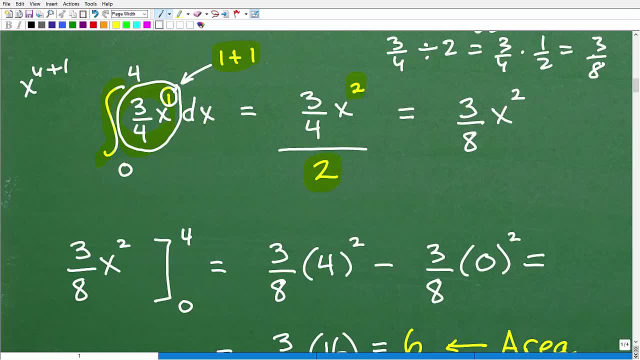 YouTube channel: uh, just check out my pre-algebra playlist. all right, so we've um, took the uh integral here. that's what we're doing, but you know, don't let this the terminology scare you. we just did, we just use this symbol and it told us to do this, okay, which got us right here. all right, so this. 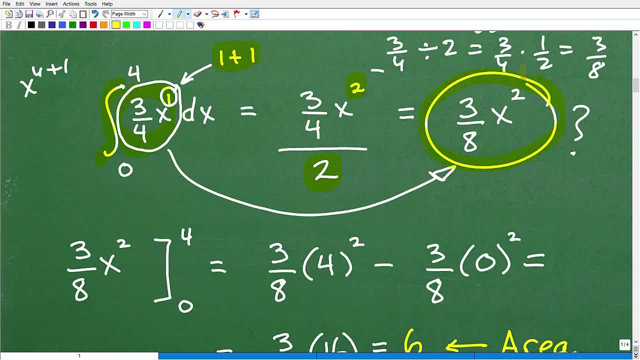 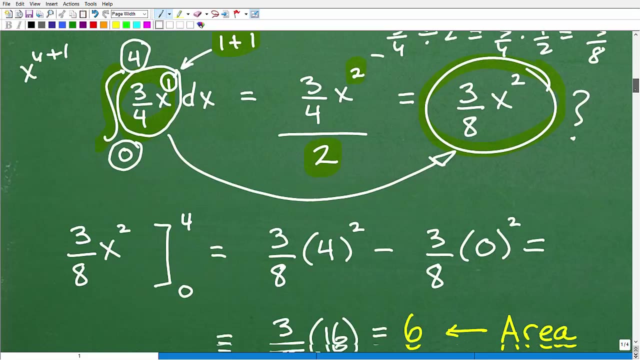 looks like that. well, this right here will allow us to actually find the area now. so, remember, we're adding up the triangle from zero to uh, four, right, so remember, over here we're going from zero to four. now, this little formula right here, this three-eighths x squared, is what will actually allow. 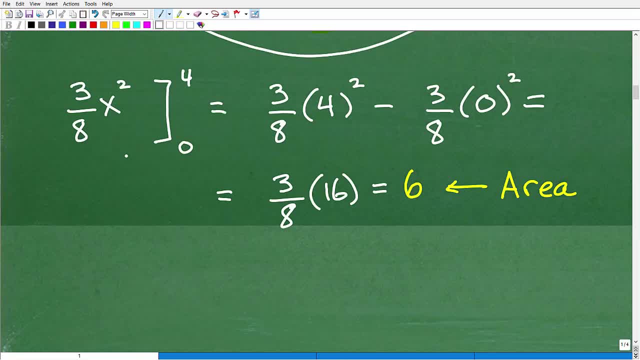 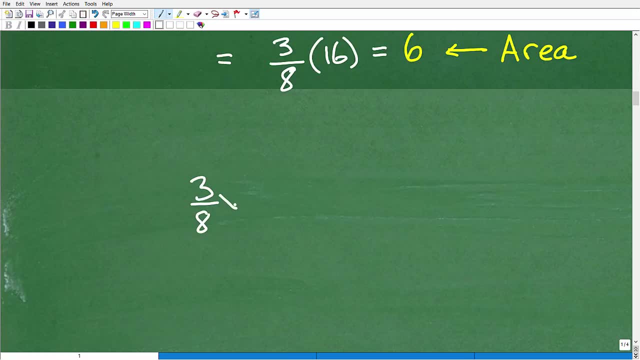 us to calculate the area. okay, so here's how it works. so we we're gonna- let me just show you right here. but we have this: three eights x squared and we're going to subtract it from three eights x squared. now, here we're going to plug in for x. we're going to let x is equal to four. all right, 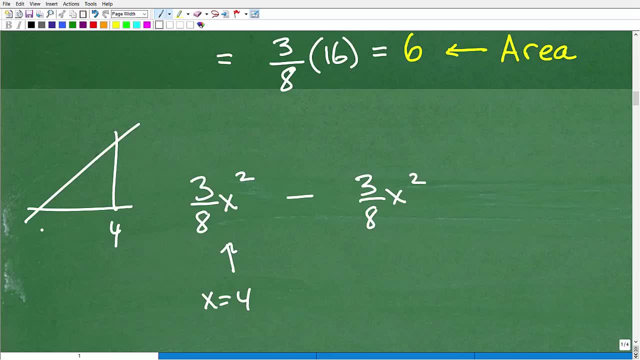 so here's a little triangle right here, so it's four and here's zero. so it kind of works a little bit in reverse. so this is going to be your ending point right there and this will be your starting point for x right there, and then I'm going to plug in four for x right here, and when I do that, 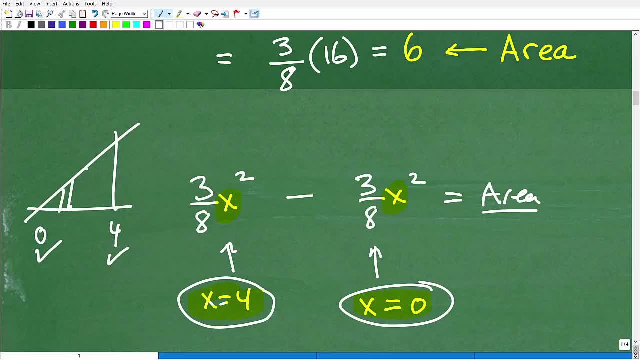 calculation. this was the area of that triangle. okay, this is, uh, this is how this works. now you can see, when I plug in zero for x right here, this whole thing will just be zero. so really what I have to figure out? what is what? three eights, um, uh, I'm going to put in four and I'm going to square. 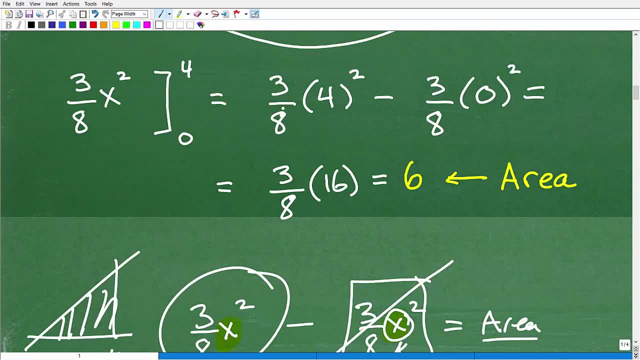 it right there. so let's go ahead and take a look at the math. I already did so. here it is. so I have three eights. I'm plugging that four squared. four squared, of course, is 16.. so eight goes into 16. two, two times three is six, and that should look familiar to you, because that is in. 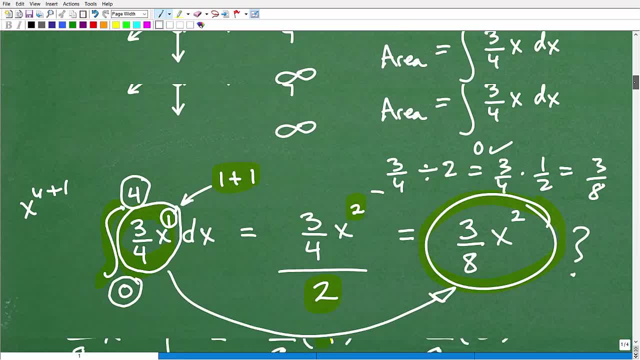 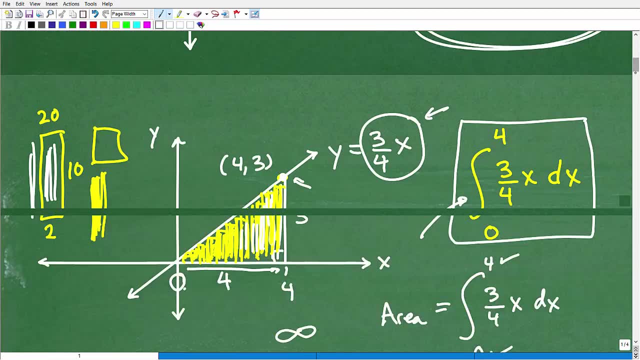 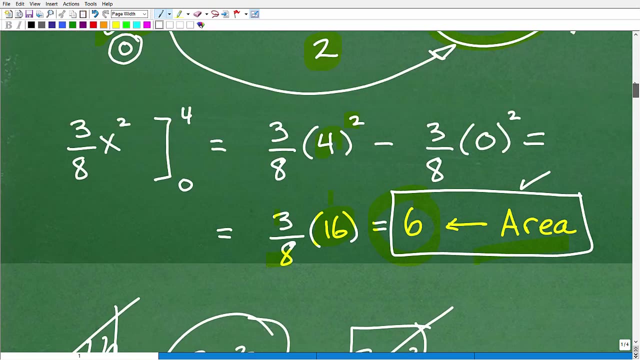 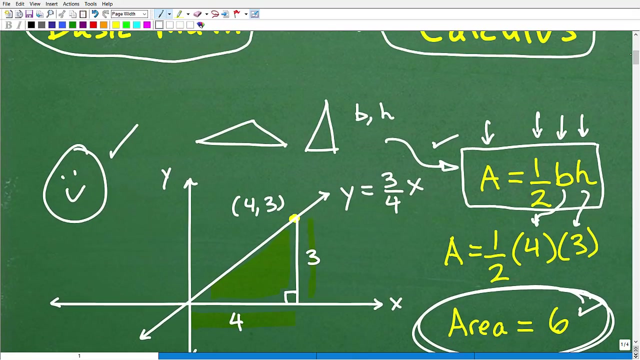 fact, the same area? answer: as when we use the formula way over here: okay, area is equal to six. but uh, you know, we obviously use calculus. now would you use calculus as a practical to use calculus here to find the area of this triangle? uh, the answer is no, okay, it would not be practical. we want to use our lovely formulas, right, so like: 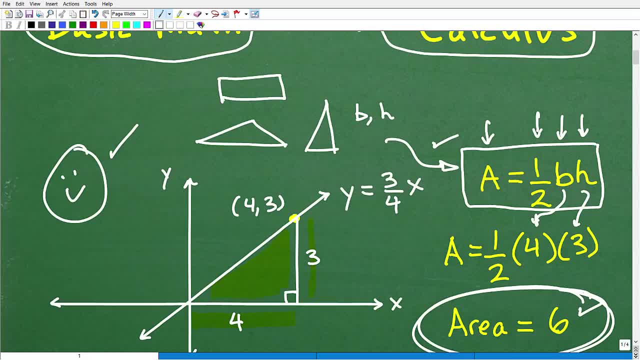 area of a circle, um, of a, you know, like a rectangle, circle, triangle, um, you know those basic figures, things like that. yeah, we definitely want to use our formula, but when we come across a thingamajiggy or some sort of crazy object and we're like, okay, there is no formula, well then we got to go ahead. 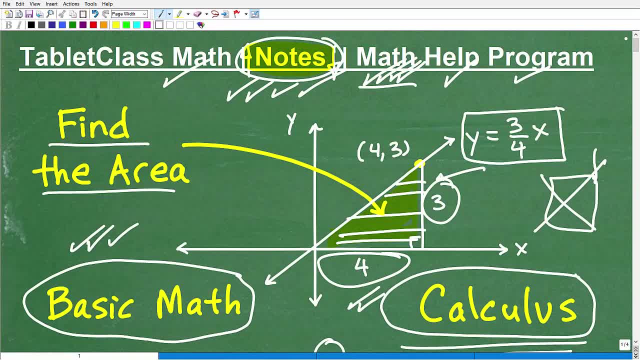 and do it. okay. so just a quick introduction of calculus and its application again, even if you- um, uh, you know, only know some basic algebra here. hopefully this video, you know, makes some sense. okay now, I would love nothing more for you to eventually one day take calculus, and it is a 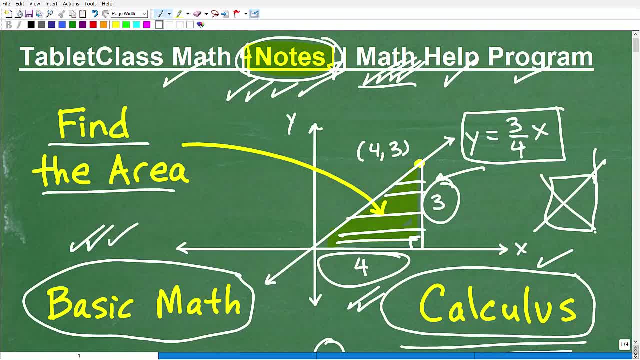 serious mathematics in terms of how advanced it is. there is, uh, you know I'm trying to minimize it and you certainly need to be ready for it because there is a lot of advanced concepts in calculus, but we could distill down the basic essence of you know um, what calculus does for us.